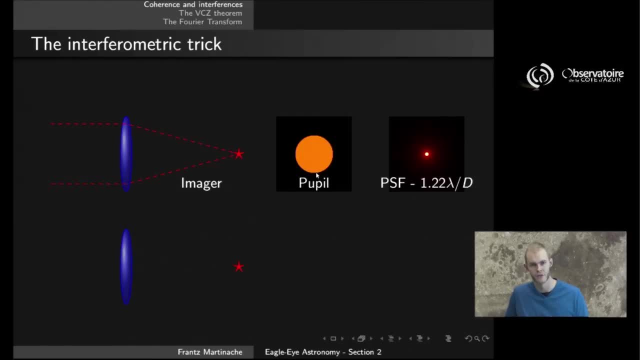 the pupil is a uniform disc of a given diameter And the image here in this case is going to be the familiar- the now familiar Airy function, which we've looked at in the previous section, characterized by a first dark ring at a radius of 1.22 lambda on D, which we've 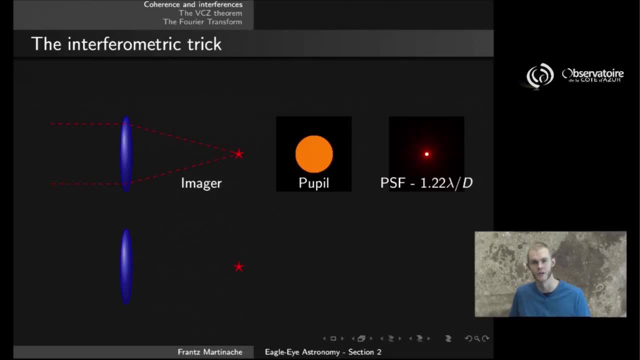 identified as being the resolution limit of our telescope. Now picture this: Let's place a mask in front of our telescope And then we're going to go to the other side of the telescope and then we're going to have our optical system within that Ricoh. 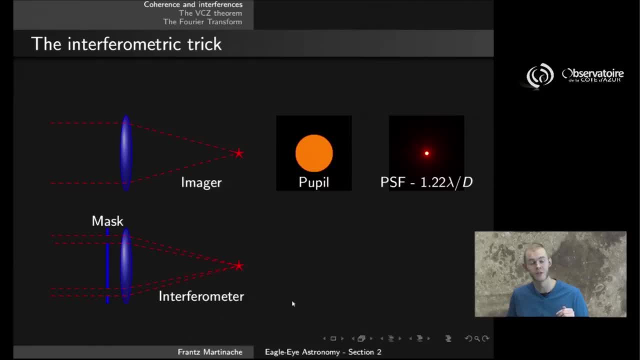 And we're going to have a pupil using a large circular aperture to observe the light into our image. And then we have the second light source, And now we have this guy, the first light source, that is, the pupil. Now let's get into the subject. 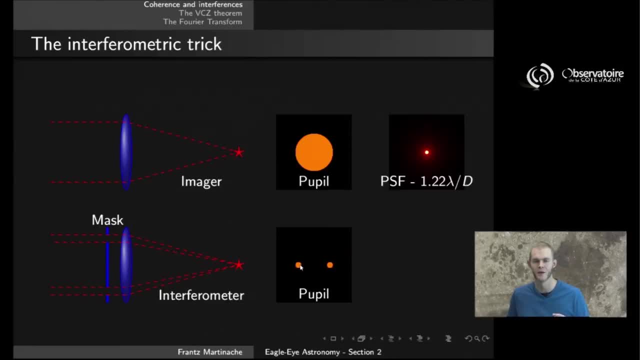 two small circular apertures separated by a distance that is comparable to the original diameter. it's a little bit smaller simply because the holes cannot be made infinitely small. the diffraction pattern produces produced by this system looks very interesting. something like that. you have a, you may recognize the. 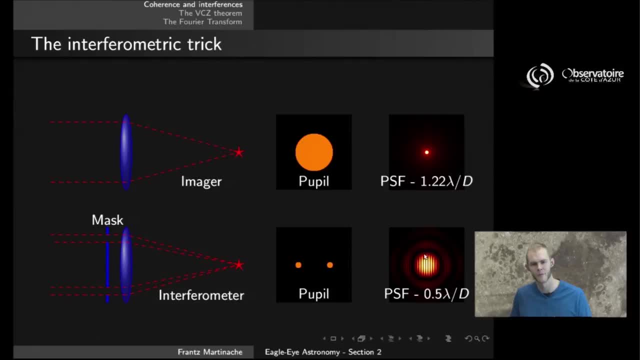 diffraction pattern of a single small aperture with a first dark ring at 1.22 lambda on D, where D in this case is the diameter of a sub aperture. but over, imposed to that diffraction pattern, you see dark and bright stripes alternating. these are we'll. we will go into refer to them as the interference fringes, as we 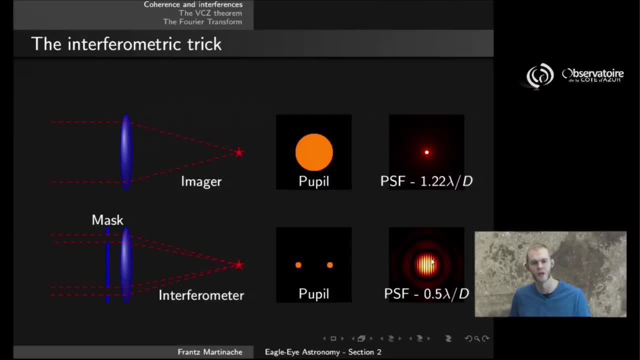 will be talking about fringes for the rest of the course and if you look at the periodicity of these fringes, you're going to see that the alternance between two dark fringes is is exactly lambda on D. that should suggest you that it is possible to access to high even if